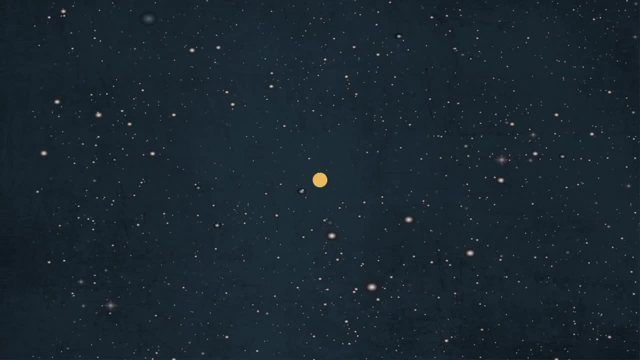 Hydrogen is easily the most abundant element in the universe. It is found in the Sun and most other stars, and the giant planets like Jupiter are composed mostly of hydrogen. On Earth it is found in water, fossil fuels and living things, but very little has the 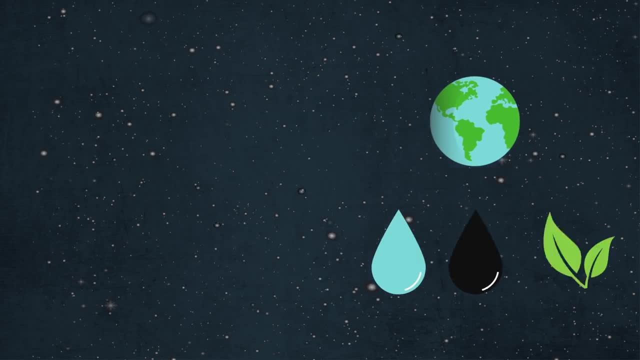 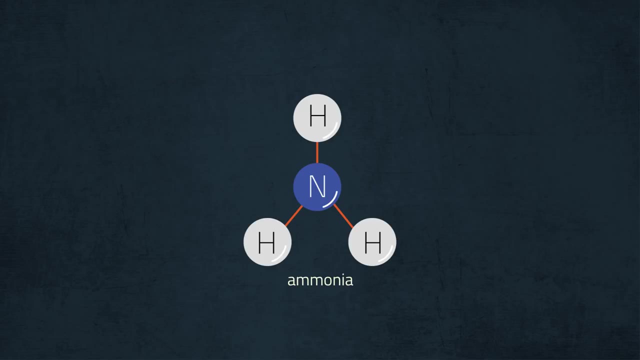 element on its own. In the chemical industry. it is used to make ammonia for agricultural fertiliser and to make cyclohexane and methanol, which are needed to make plastics and pharmaceuticals. It is also used to remove sulphur from fuels during the 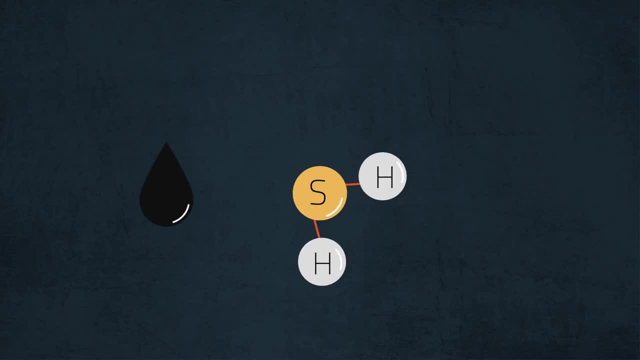 oil refining process when it forms the bad egg-smelling gas, hydrogen. Hydrogen sulfide. Large quantities of hydrogen are used to hydrogenate vegetable oils, to form fats, for example to make margarine. The H in the pH scale denotes hydrogen. It represents the concentration of hydrogen ions. 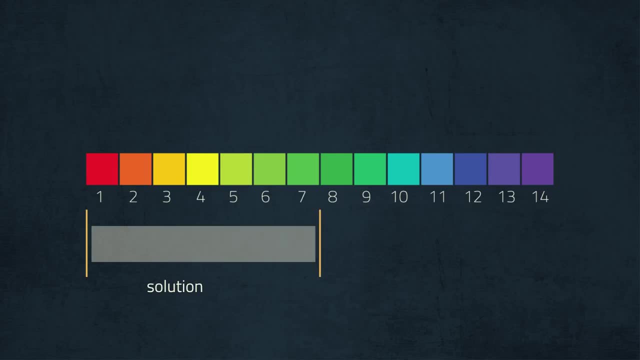 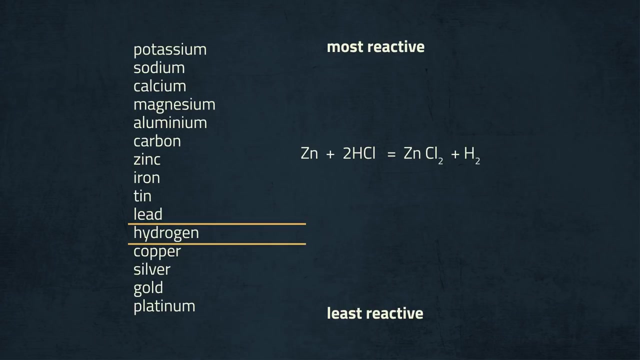 in water When the pH is lower than 7, the solution is acidic and it is the hydrogen, or more strictly, the hydroxonium ion that makes the acids react. Thus, metals above hydrogen in the reactivity series normally react with acids to form hydrogen. 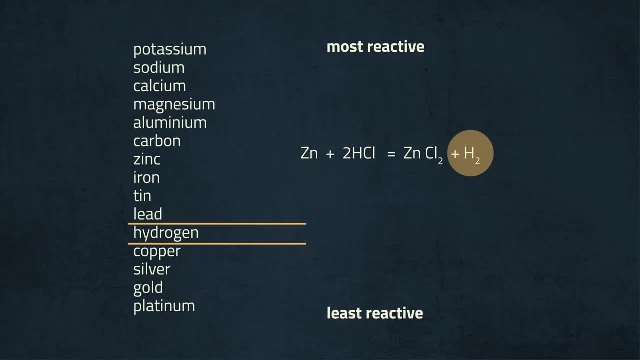 like zinc with hydrochloric acid. However, if the metals form an insoluble salt, little reaction will occur. for example, lead in sulphuric or hydrochloric acids. Aluminium metal, although well above hydrogen, is covered with a tight layer of oxide which 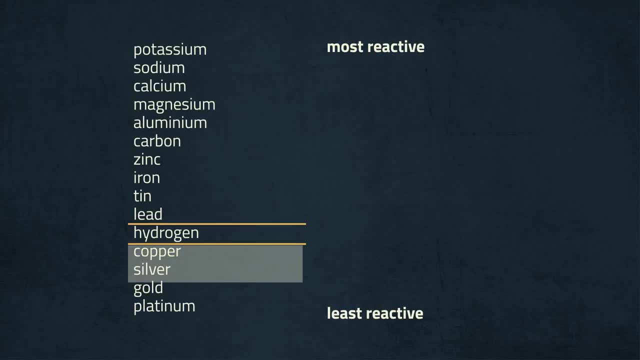 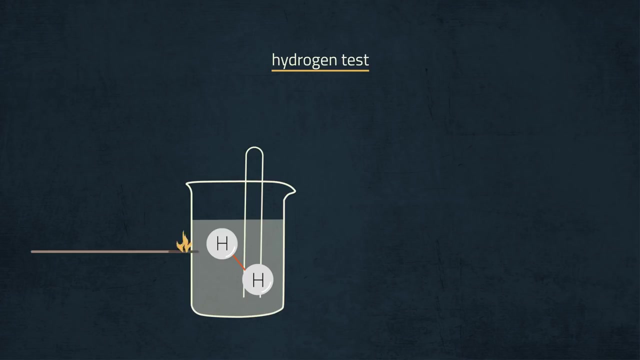 protects it from acid corrosion. Unreactive metals below hydrogen do not displace hydrogen in acids. The most reactive metals will react with water itself- sodium, for example. You can test for hydrogen by exposing it to a flame. It ignites with a squeaky pop and 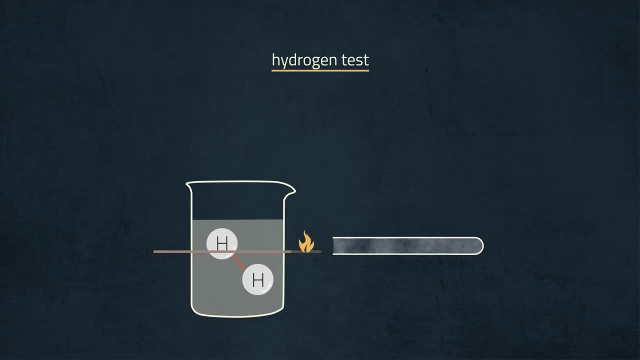 you can see condensation in the tube as water is formed. Although hydrogen is an essential element for life, it doesn't play a particularly active role. It remains bonded to carbon and oxygen. In addition, the nitrogen in oxygen is attached to the oxygen atoms, whilst the chemistry